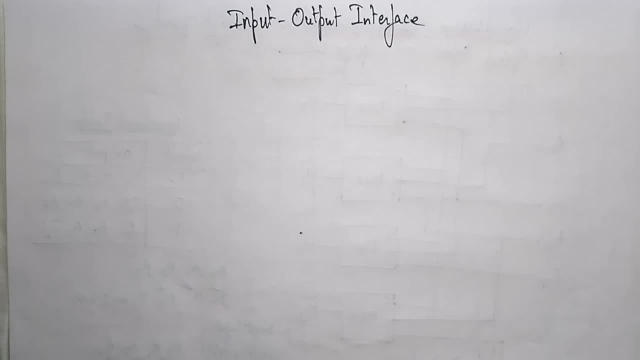 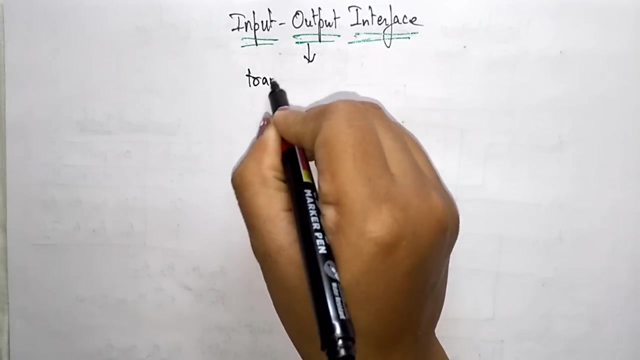 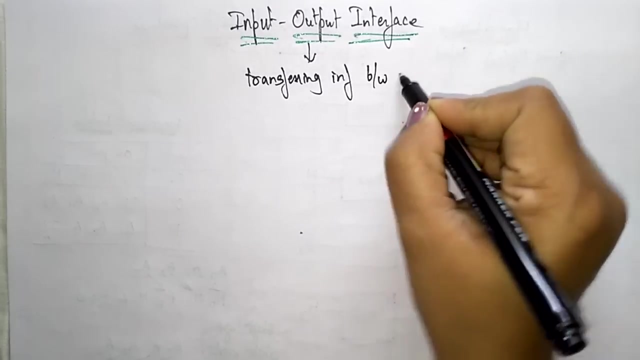 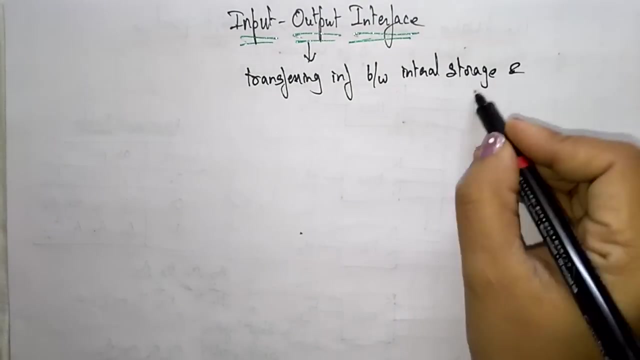 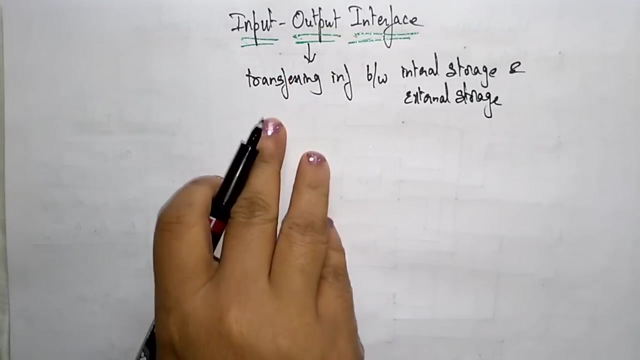 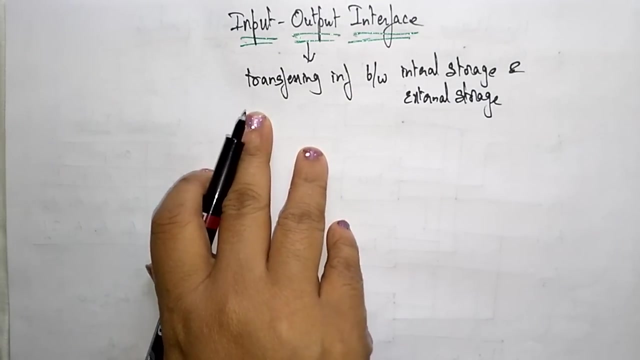 Hi students, coming to our next topic, that is, input-output interface. So what is this input-output interface? This IO interface provides a method, So it provides a method for transferring information between internal storage and internal storage And external storage. Okay, So this input-output interface? nothing but it provides a one method. So that method, what that method will do? It transfers information between internal storage and external storage. 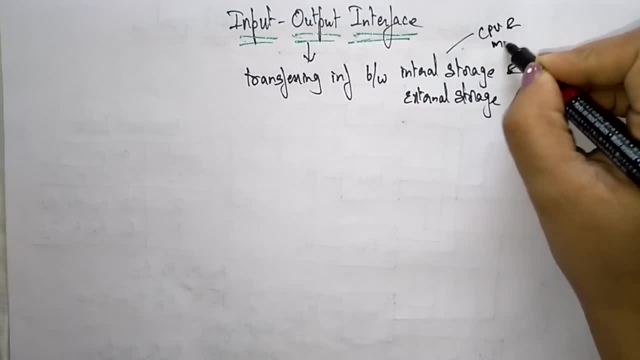 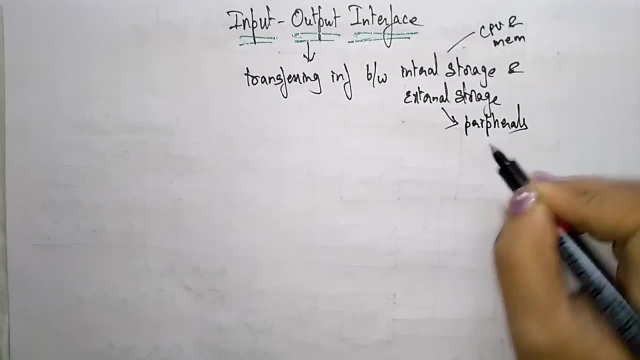 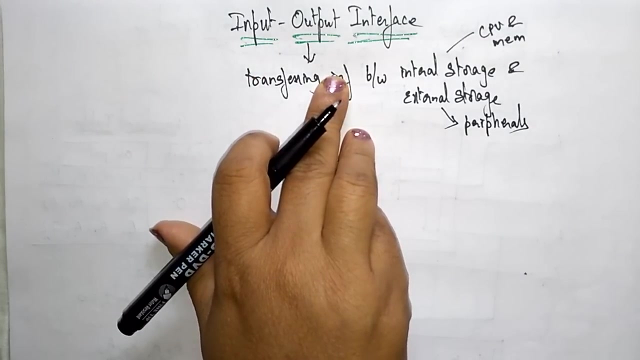 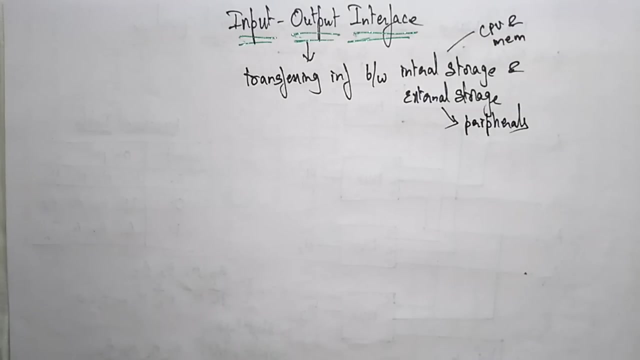 Internal storage, or nothing but the CPU and memory. you call it as internal storage. And external storage means all the peripheral devices Which are connected outside the system. Those are called the external storage. So a communication between the CPU and memory and peripheral devices. One interfacing circuit will be there, That is the input-output interface. Actually, in order to interface peripherals with the CPU, a special communication lines are required. So to communicate the CPU, 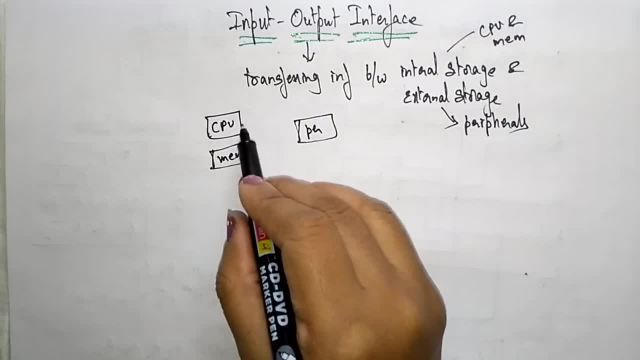 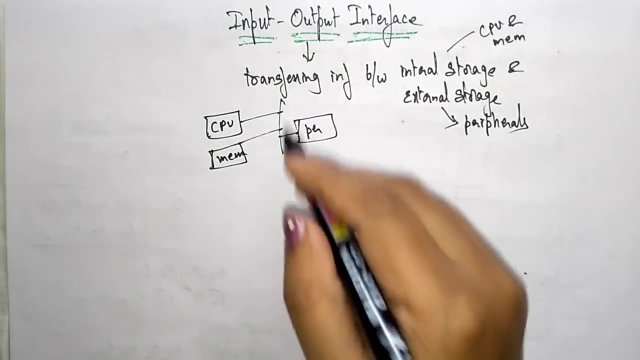 Peripherals. So for all this some communication lines are required. Okay, So you call it a special communication lines. So it also resolves the difference between the computer and peripheral devices. So, whatever the special communication lines, So you call it as some input-output interface. So this input-output interface resolves the difference between the computer and peripheral devices. 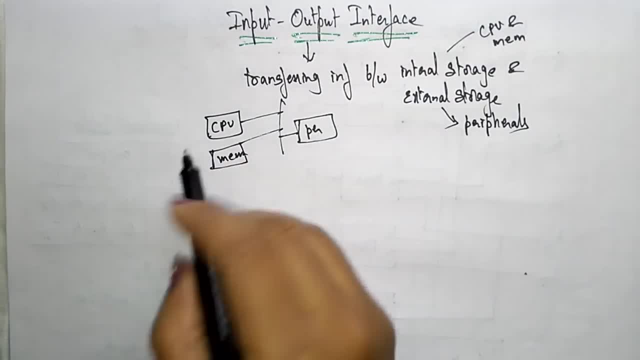 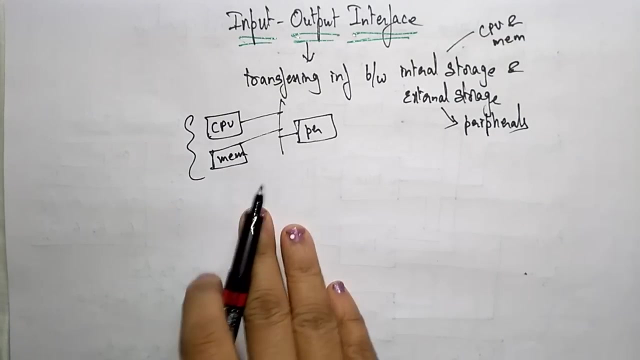 Interface Versus the difference, The Computer Interface, internal storages and the peripheral devices. How it results. first, know the difference between these peripherals and the CPU. So why we required one input output interface to communicate the data transfer between the peripherals and the CPU. 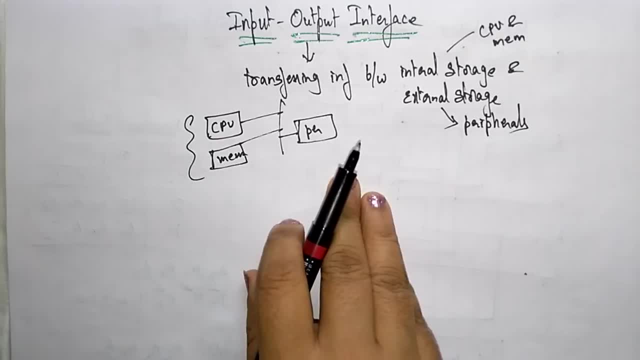 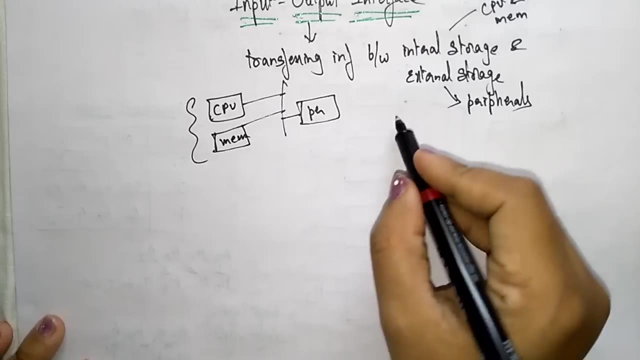 Why we can't directly move the data from peripherals to CPU and from CPU to peripherals, Why we required one extra input output interfacing circuit. So let us see why we are going for this input output interface. First, see the difference between the peripherals and the CPU. 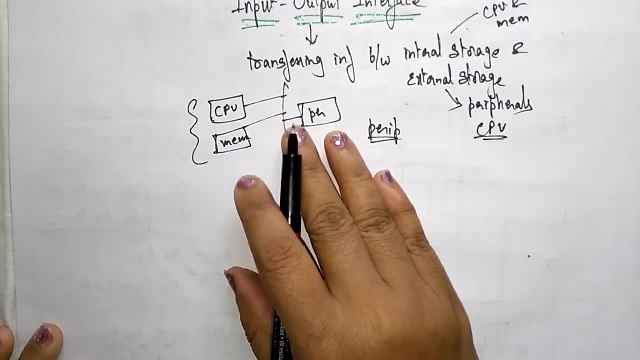 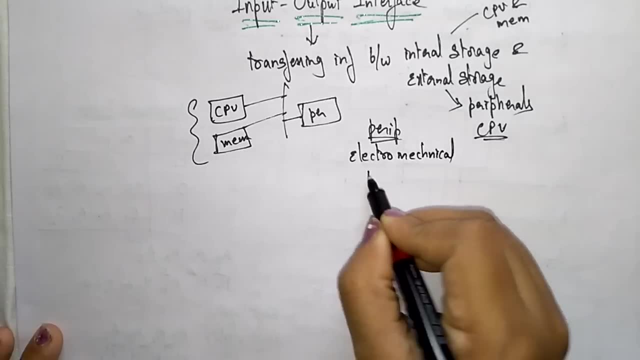 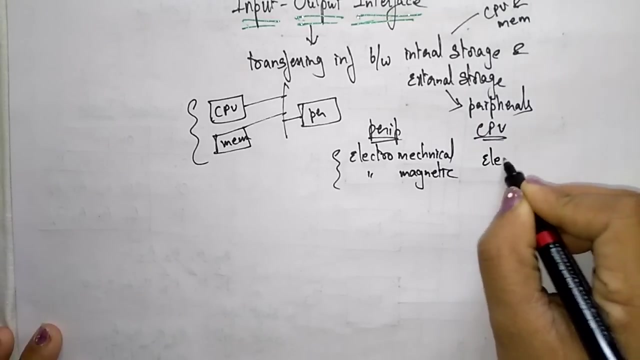 So actually the all the peripherals, what are connected to the system or Electro, and the Electro-mechanical or Electro-magnetic devices. So the peripherals that are connected to the systems or the Electro-mechanical and Electro-magnetic devices will be connected, Whereas the CPU is electronic device. 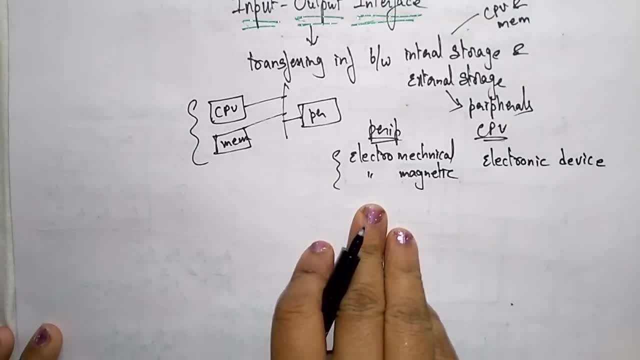 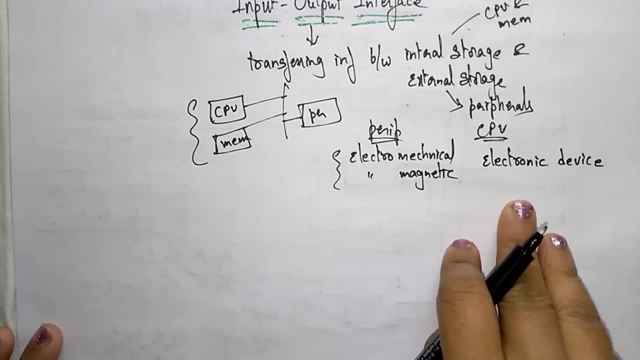 So this is completely different. It is Electro-mechanical whereas it is- this is electronic device, So a communication between these two. So this is electronic device, So a communication between these two. So the communication between this peripherals and the CPU is somewhat different, because 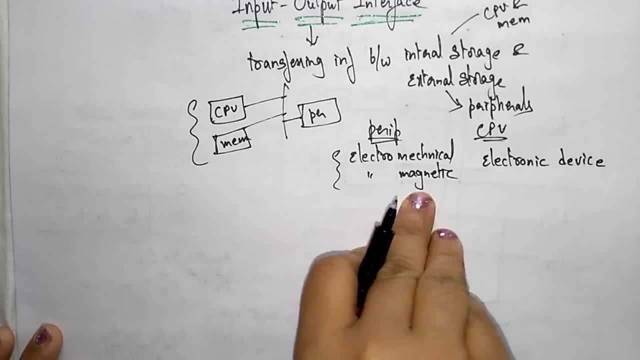 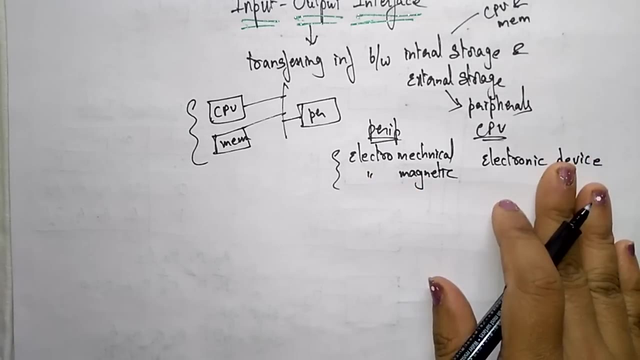 they can't directly communicate. mechanical devices will not directly communicate with the electronic device, So to communication between these two, one interfacing circuit will be required to change the main. suppose these people are speaking in one language and these people are speaking in another language. Okay, so if they do, they want to communicate to each other. 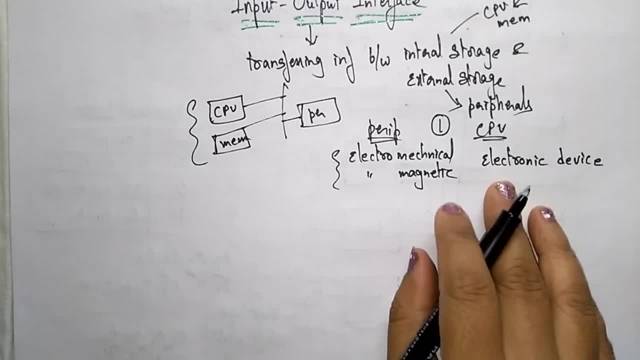 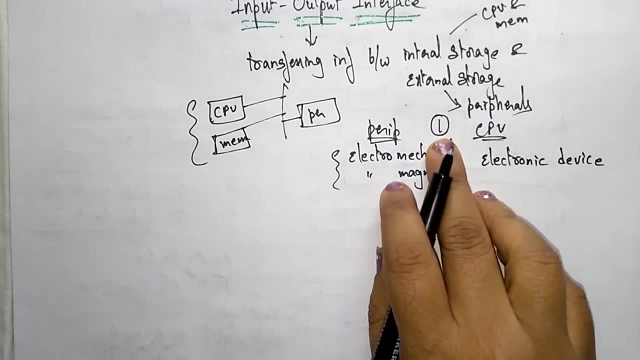 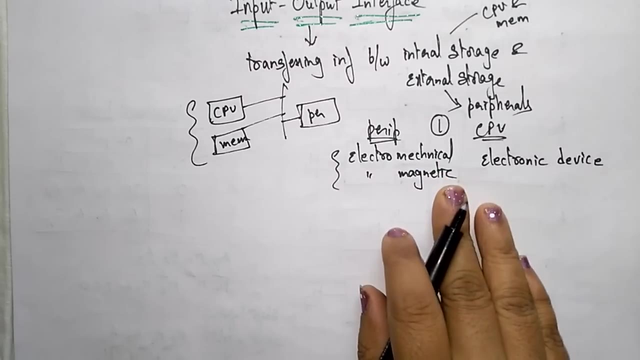 So this person has to be, acts as an intermediate between these two people to communicate. So this person will tell in his language and this person will communicate to in his language means the conversion. So like that an input output interfacing circuit will require to communicate between the peripherals. 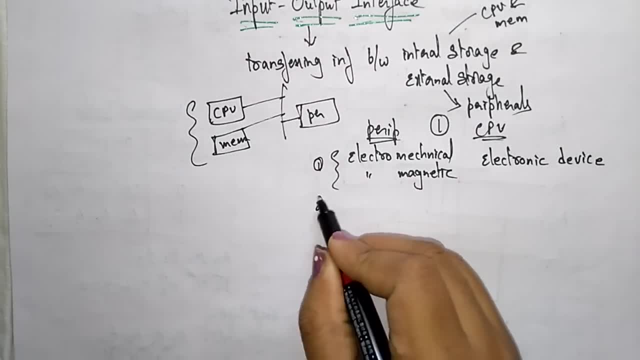 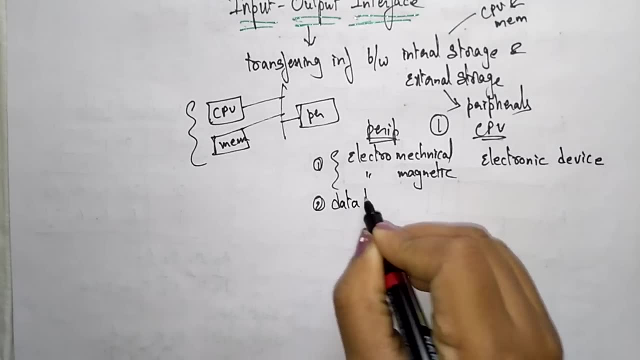 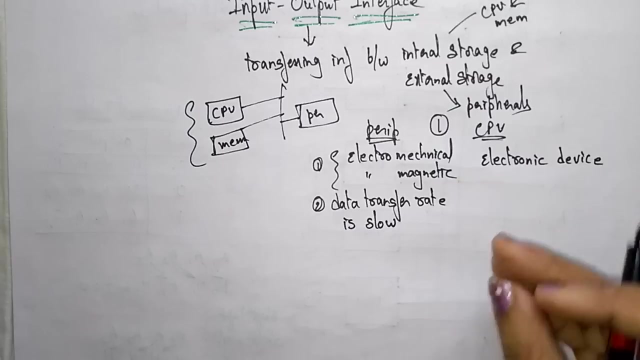 and the CPU. and one more difference is this: peripherals or the data transfer rate is slow. Here data transfer rate is slow when compared to the CPU, So all the peripherals are sending the data very slowly when compared to the CPU. So the CPU can't wait until the peripherals is sending the signal, means the CPU wastage. 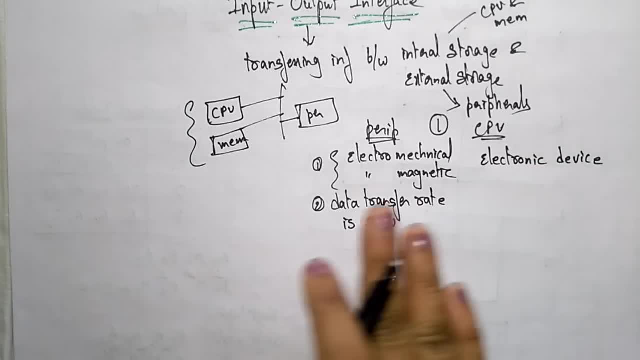 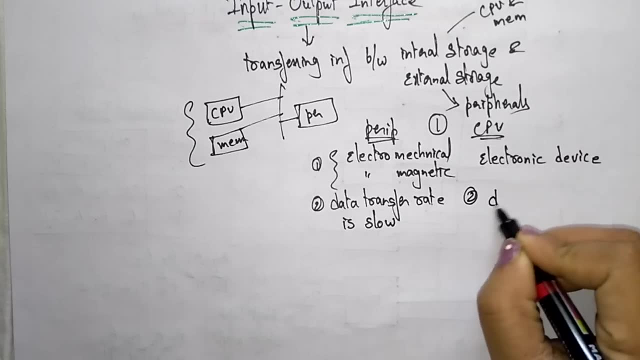 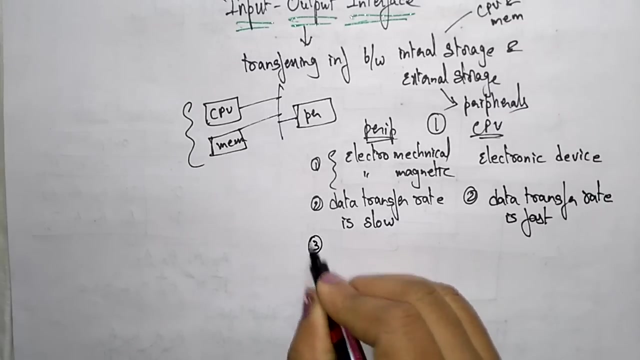 time is increasing, So it has to be wait until the peripheral is sending the data. Okay, so this is one of the difference Here. the CPU is data transfer rate. Data transfer rate is rate is high, is fast when compared to the peripherals. So this is one more difference between those, these two. 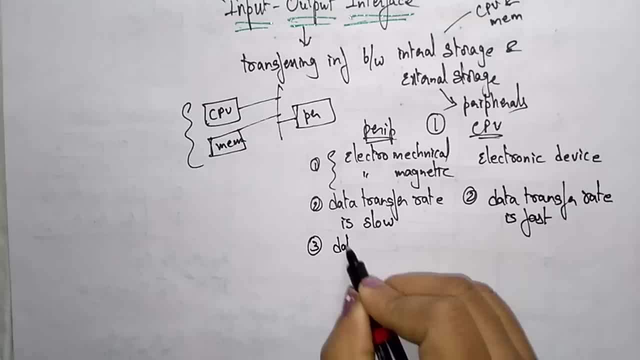 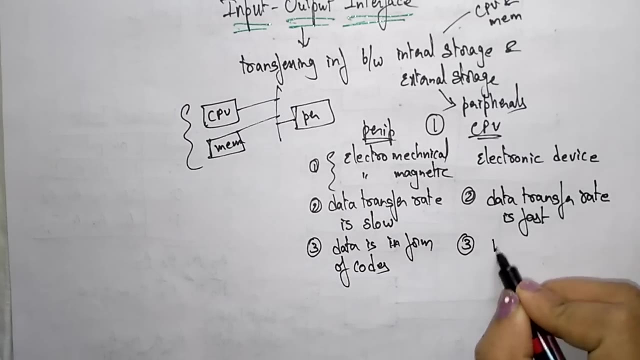 And the third difference: here the data data is in the form of codes, So all the data that is in the peripherals is in the form of codes, Whereas in the CPU the data is in the form of word. So the CPU can take the data word at a time, but whereas in peripherals it is in codes. 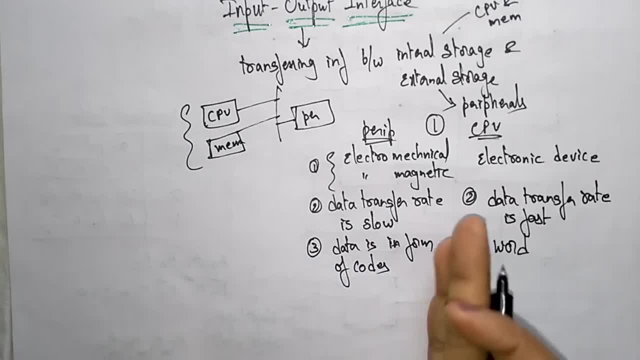 So to convert the codes into word we need some interfacing circuit, that is the input output interface. So this input out to output interface resolves the difference between the computer means, the CPU, and the peripheral devices. So the main use of this input output interface is to resolve the difference between the CPU. 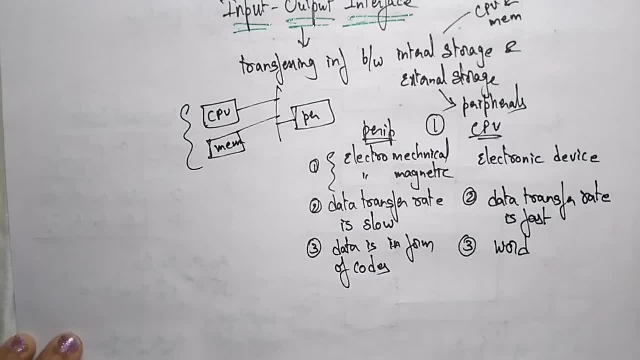 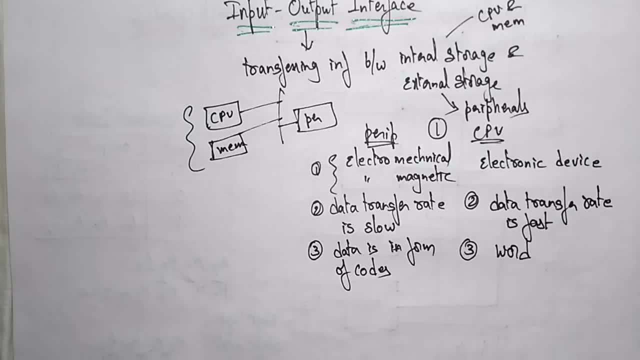 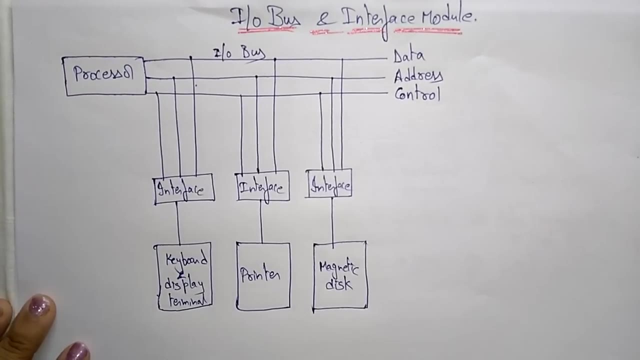 and the peripherals. we require one interfacing circuit. So let us see IvoBus and interface module. So this is the IvoBus and interface module- Actually, these IvoBus and interface modules- synchronizes the data flow and supervises the transfer. 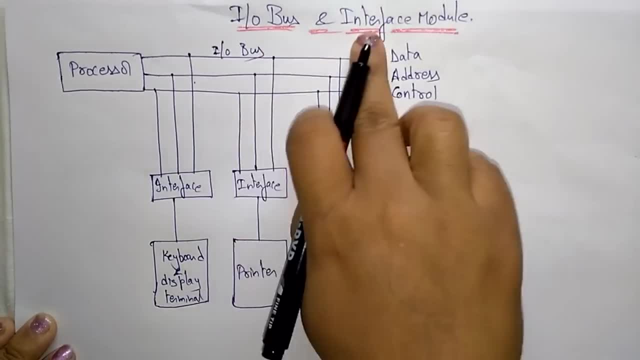 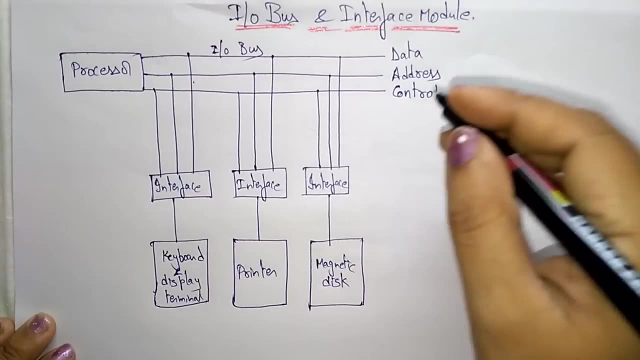 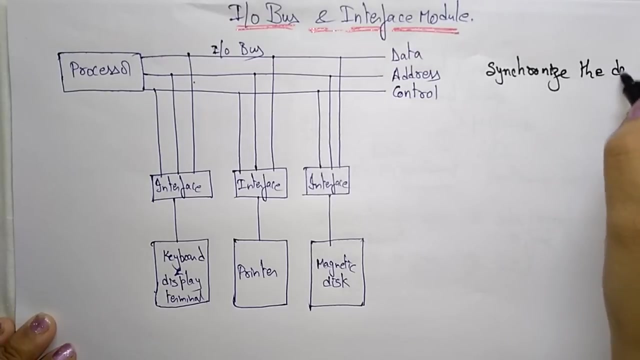 So its average transfer rate between the peripherals and processor means why we are using this IvoBus and interface module between the CPU and the peripherals: because it synchronizes the, It synchronizes the data flow. so I already said okay, I already said the peripherals are. 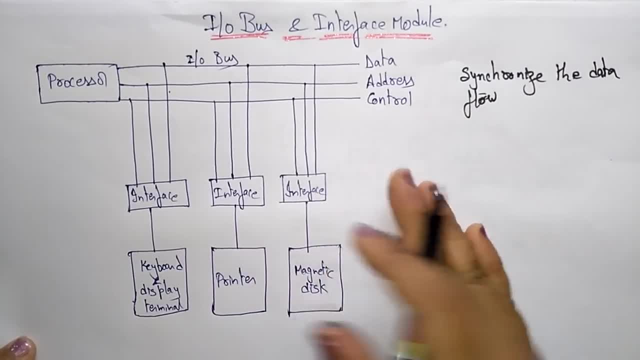 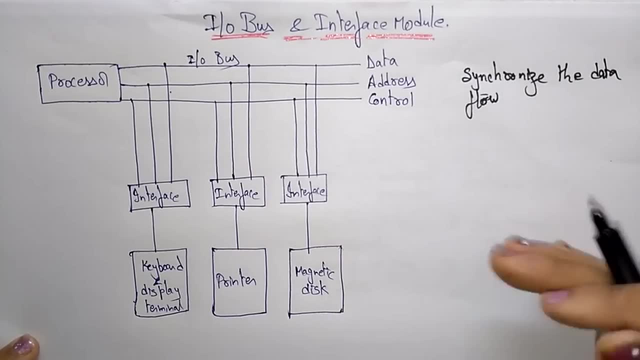 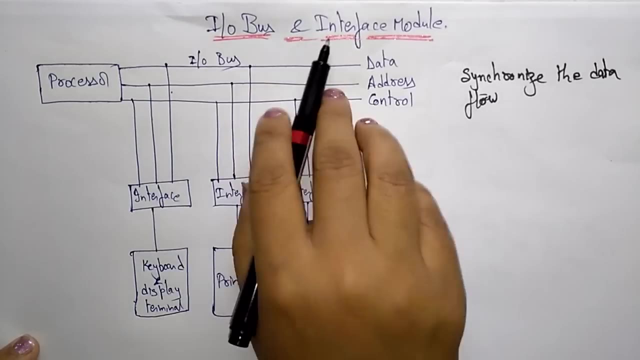 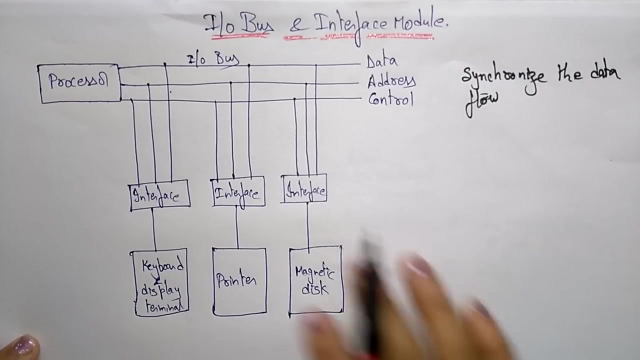 sending the data very slowly, whereas the CPU is data transfer rate is very fast. their communication, to make them mutual understanding, to synchronize the communication, to synchronize the data flow, we required iobus and interfacing module between those two devices. okay, and also it supervises the transfers between the peripherals and the processor. so this is the 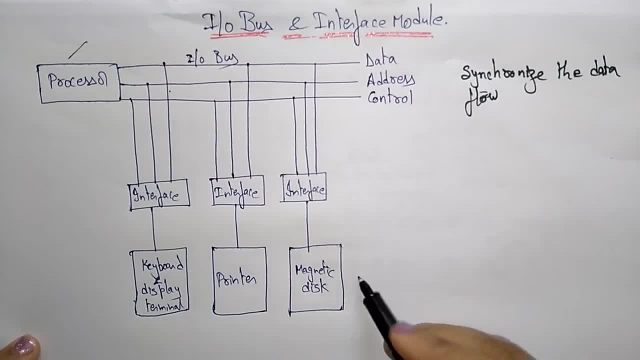 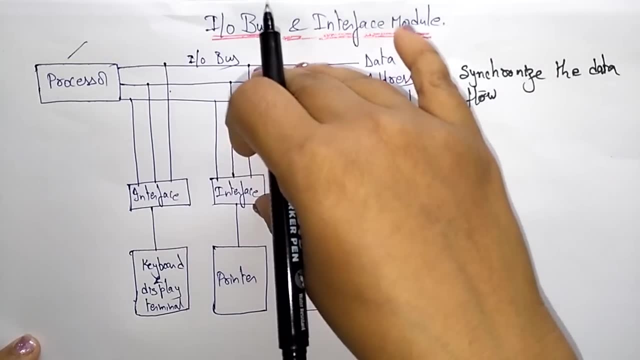 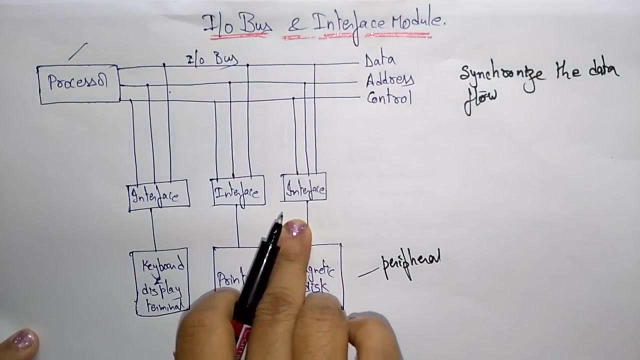 processor, the cpu, and these are all the peripheral devices. these are the peripheral devices, so the cpu and the peripheral devices. in between this we are connecting iobuses and the interface modules. i o interface modules. okay, so these are the special communication lines used to convert the data. 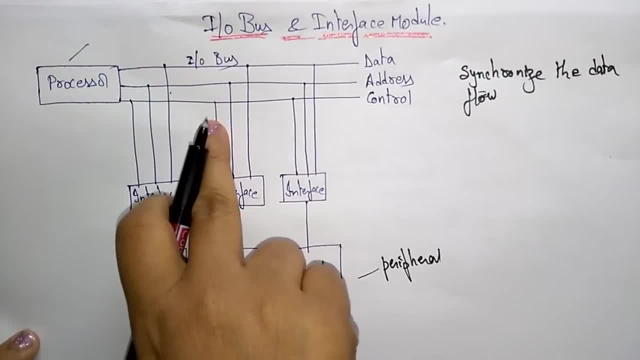 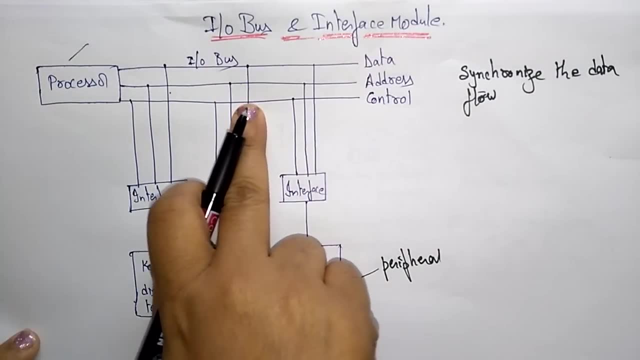 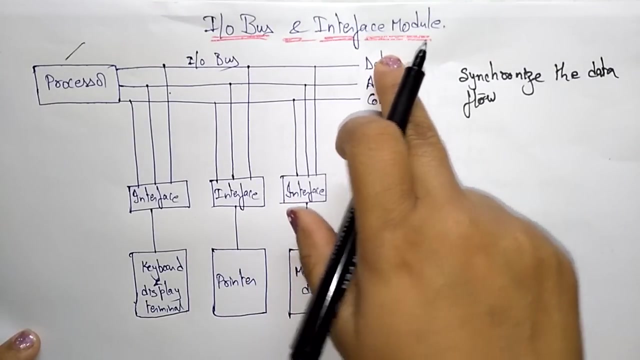 or whatever it may be. uh convert the information to the peripheral devices and from peripheral devices to the processor. so this iobus is nothing, but it is having the data bus, address bus, control bus. data bus is using the to hold the data of the information data and address bus is used to hold the address and. 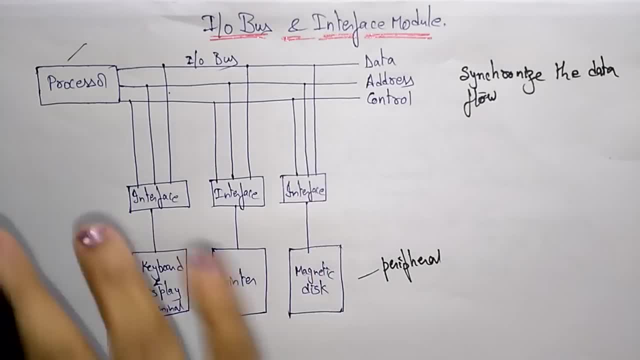 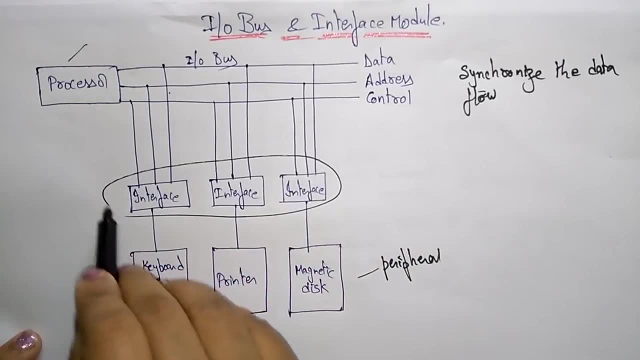 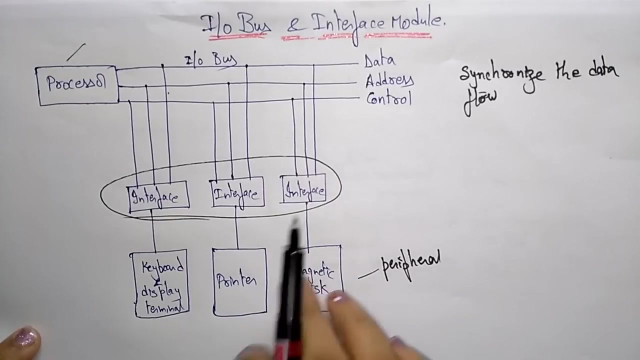 the control bus will pass the control signals from one device to the another device. so in between the processor and the peripheral devices you are having interfacing circuits. so these are the interfacing devices. so these interfacing device is used to convert, it is used to synchronize. 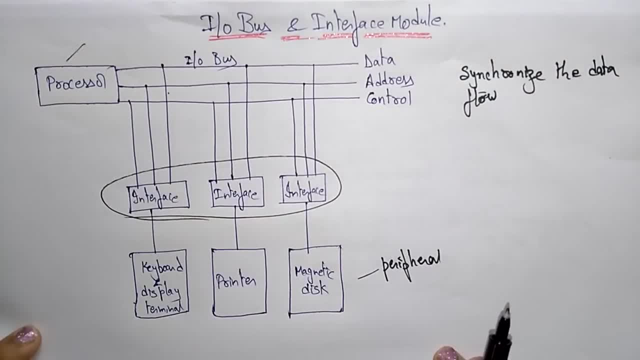 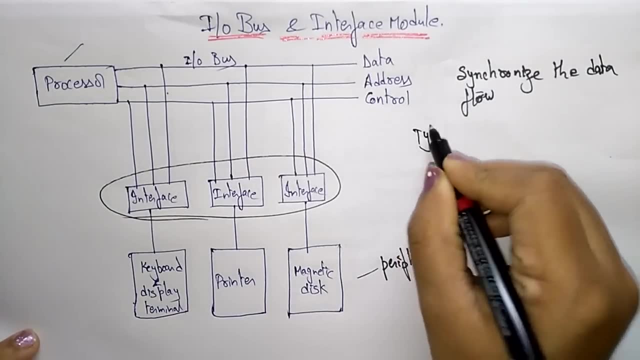 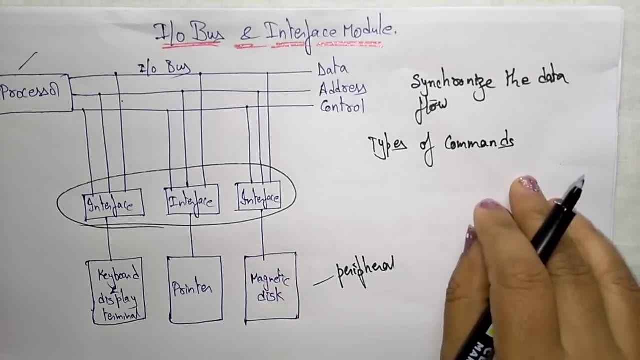 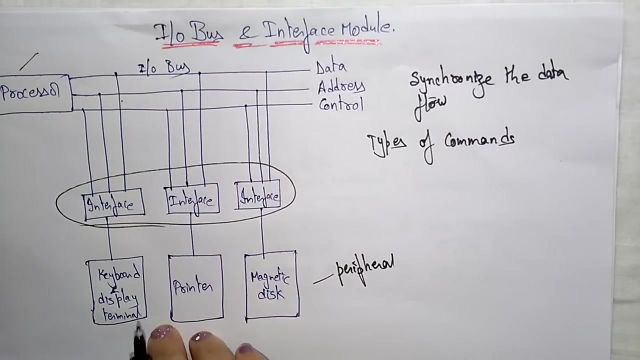 the data flow between the peripherals and the processor. so here you are having the some, some types of commands. let us see types of commands in iobus and interface module. so iobus and interface module has to be communicate with the processor and the peripherals with the help of these commands. okay, let us see first. 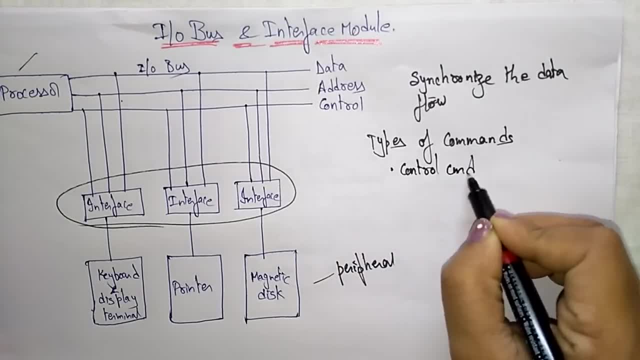 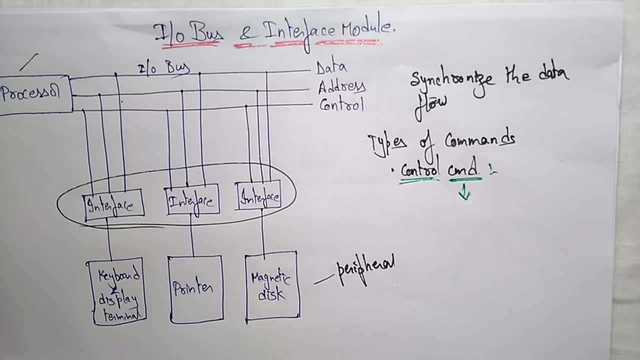 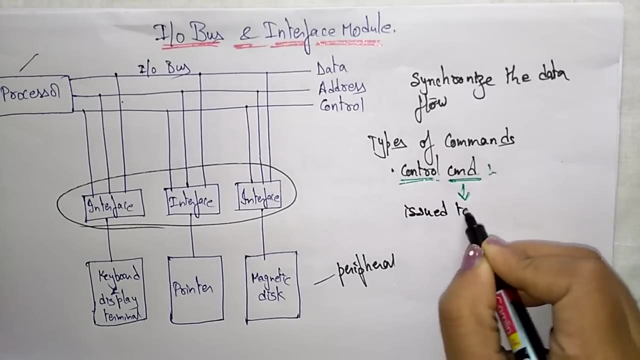 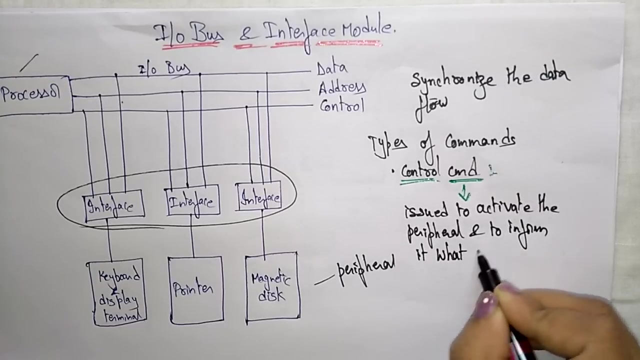 command is the control command. so what this control command will do. okay, so what this control command will do. actually, this control command issued, this control command is issued to activate, to activate the peripheral and to inform, inform it what to do. okay, so what the control command will do. the control command issued to 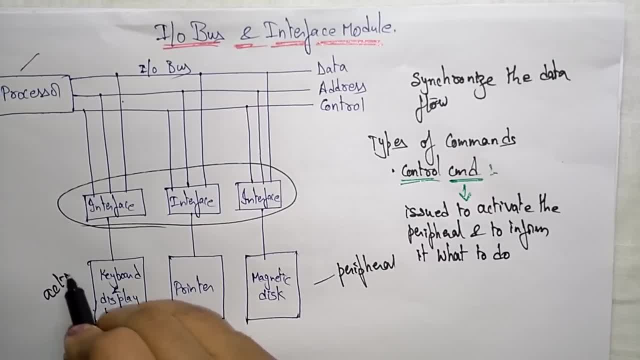 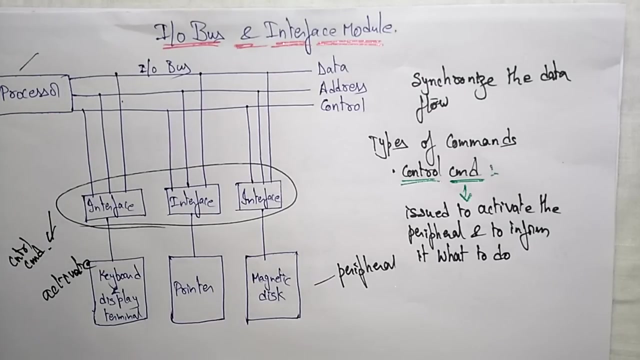 activate the peripheral. it activates the peripheral, okay, and also it tells to in peripherals what you have to do. so this interfacing circuit issues the control command, issues the control command to the peripherals, okay. so what it is issuing, it's saying that you have to be activate and you have to do something. so what you have to do, that will be tell by this. 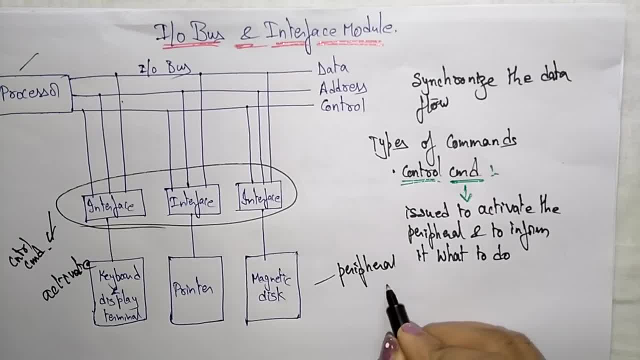 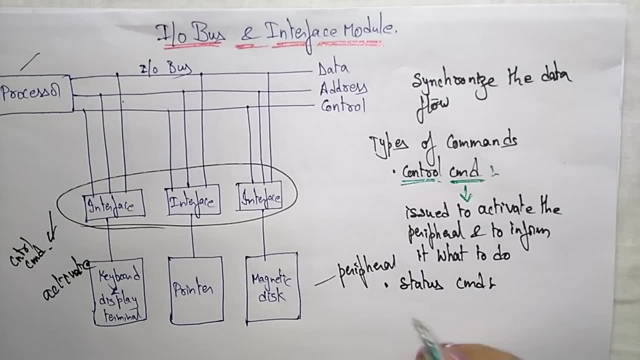 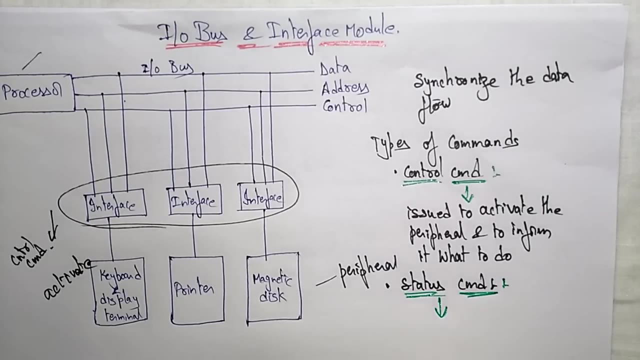 interfacing circuit to the peripheral devices. so next, coming to the next command word, so that is a status command. okay, so what's the status command will do so. actually, status command is used to test various status conditions. it is used to test various status conditions. okay, so it is. 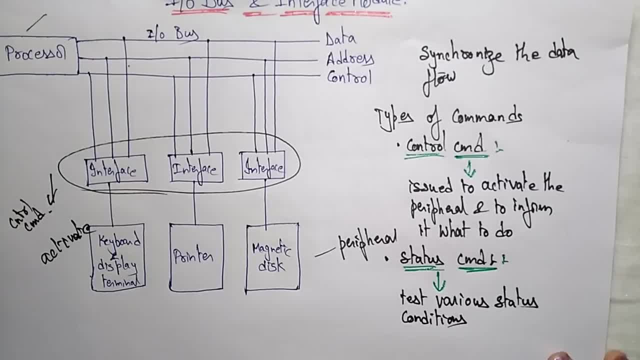 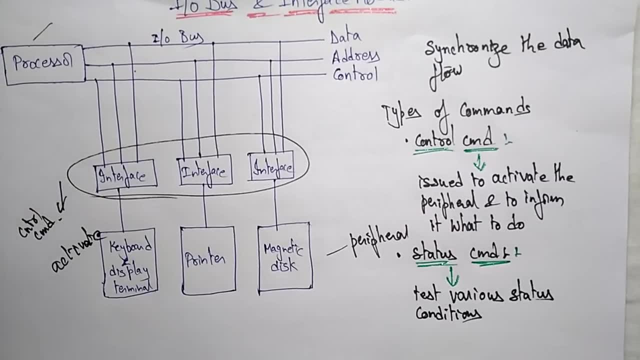 going to be test conditions, different conditions, uh in the interfacing circuit. so whether the peripherals are active or not, whether when we have to send the data, so which stay? which status is it in? so it test all the various status conditions, uh with the help of the status. 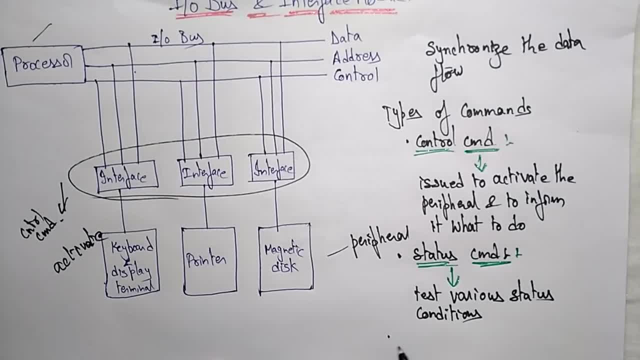 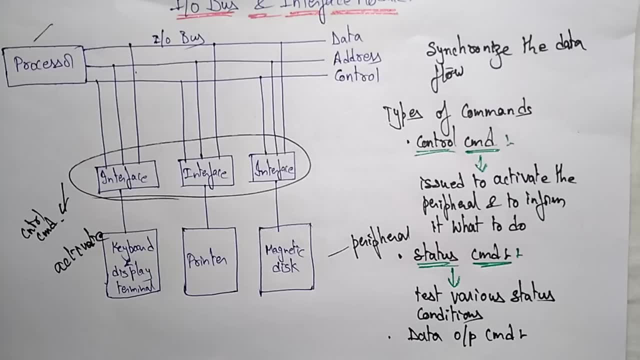 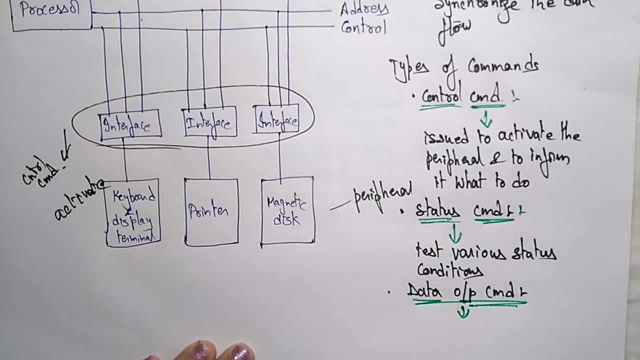 command, so next command, so next is data output command. okay, so next is the data output command. so what this data output command, uh will tell to the processor and the peripherals? actually this: it causes the interface to respond by transferring data from bus into one of its register output. so 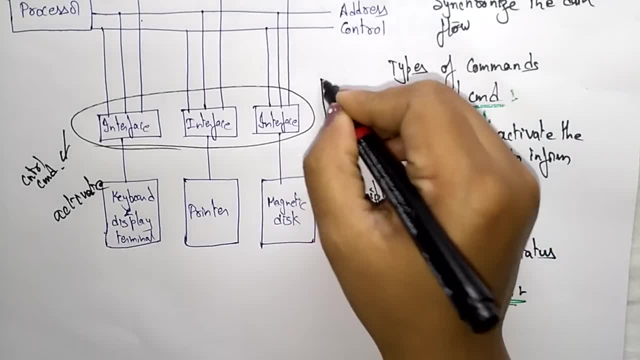 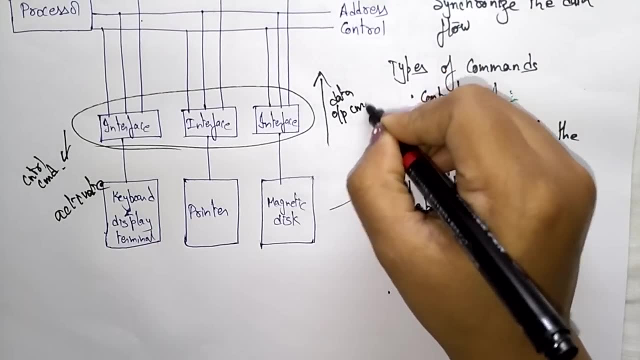 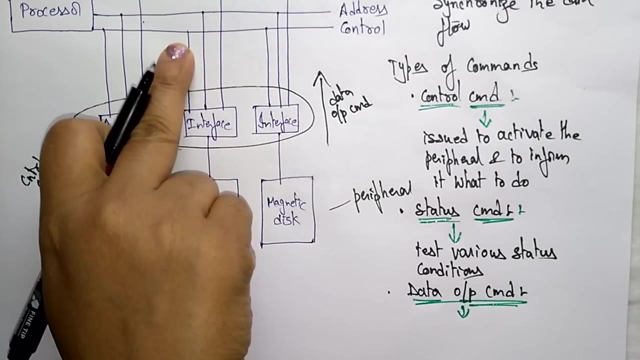 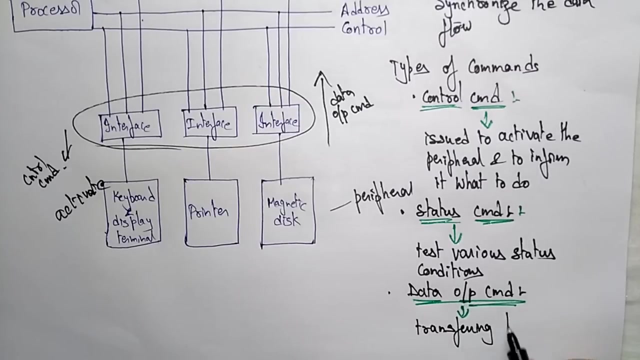 to where output. so this uh from peripherals to processor. so this: we use data output command, so interfacing circuit. uh sends the information to the processor. so what type of information it is uh sending to the processor? it transferring data from bus, so from bus, into one of its registers. so one of its registers. so data output command. 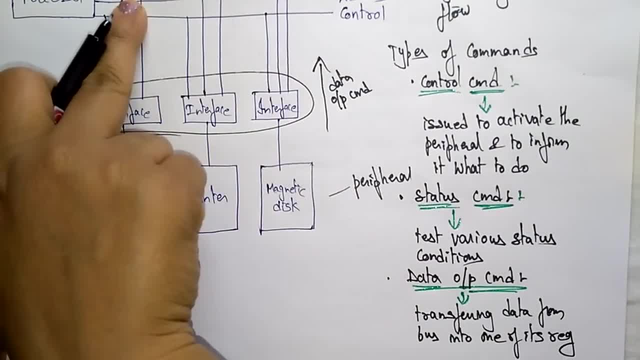 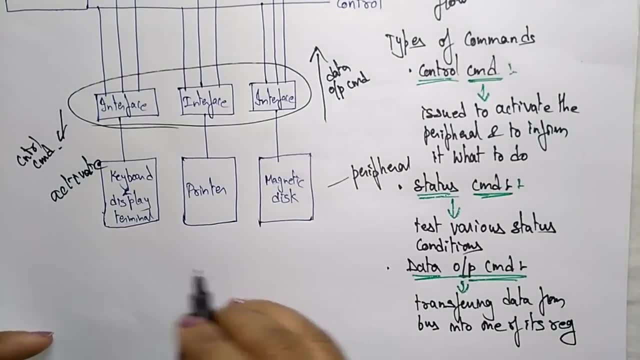 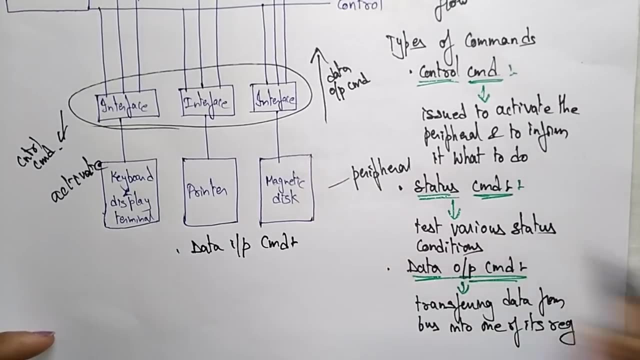 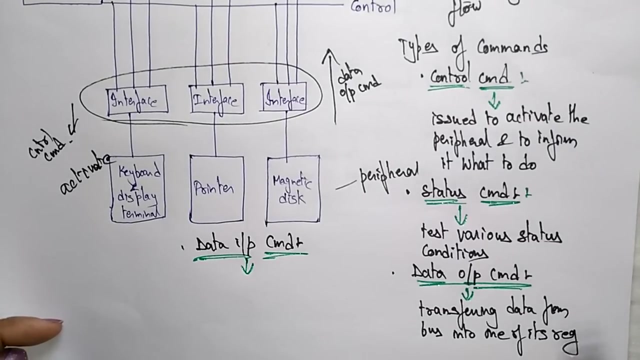 transferring data from buses to one of its output, uh, one of its registers which are present in the process. so that is one, uh, one type of command. next, data input command. okay, so what this data input command will do? so, data input command, so input command itself is saying: this is from interfacing to 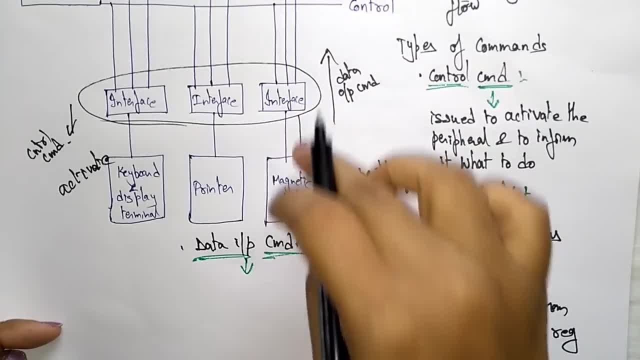 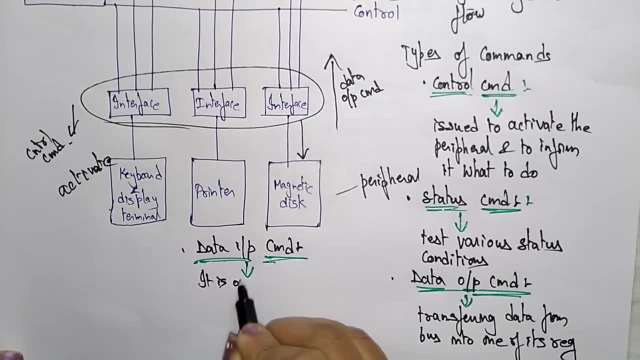 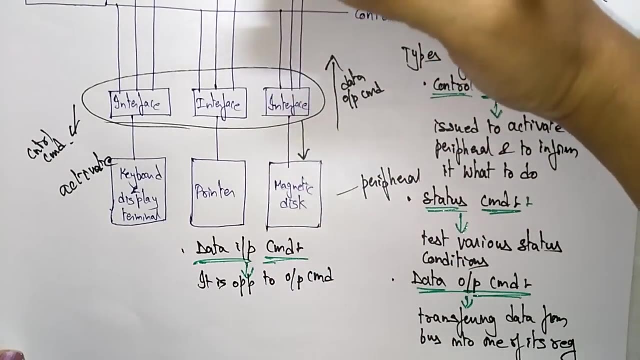 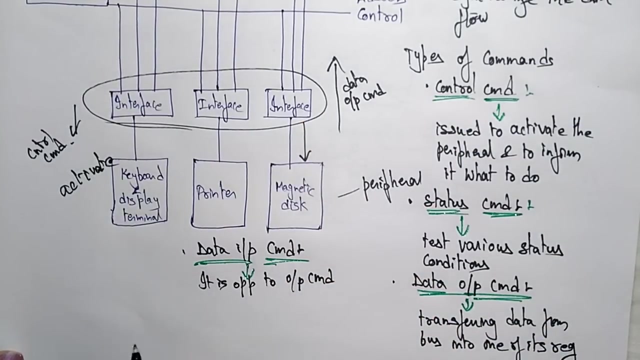 peripheral devices. so it is giving some uh information to the peripheral devices with the help of data input command. so it is just opposite to opposite to output command. so here it is sending data to processor and it is just opposite to uh output command. so in this case the interfaces receives. on item. 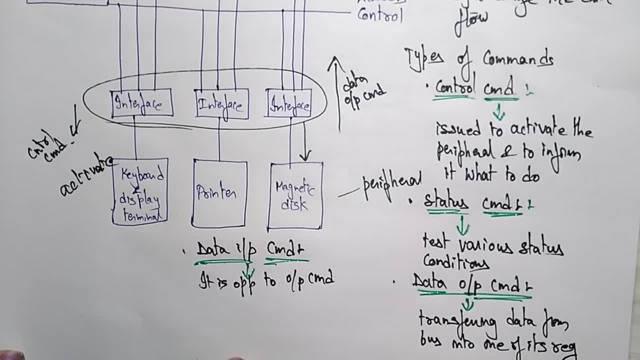 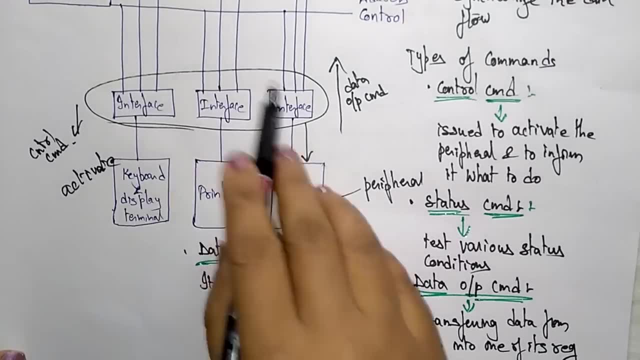 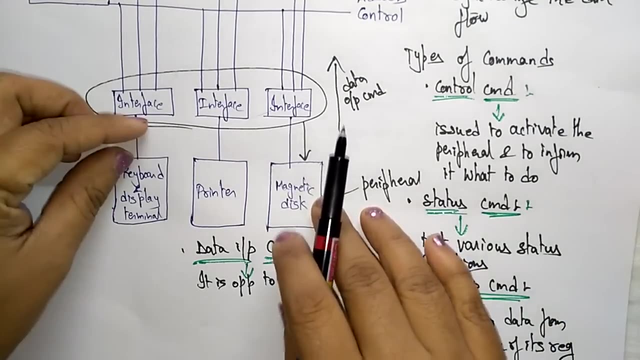 item of data from peripherals, and peripheral data has lifetime access to items on the interface. so place it in its buffer registers. so it's just taking the in, in this case the interfaces. these interfaces receives the data from peripherals and places it's in buffer, so it's a this interface here. this is the input. 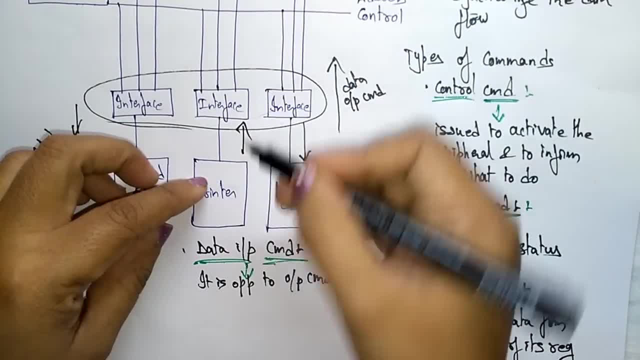 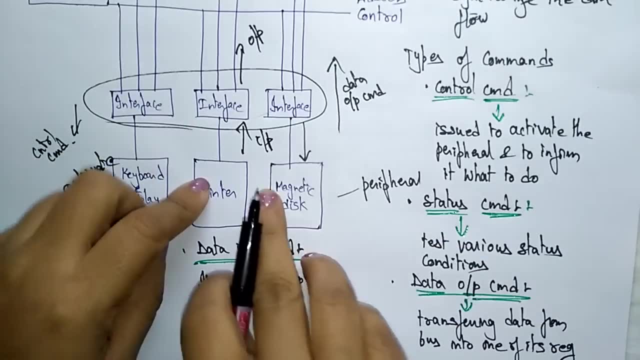 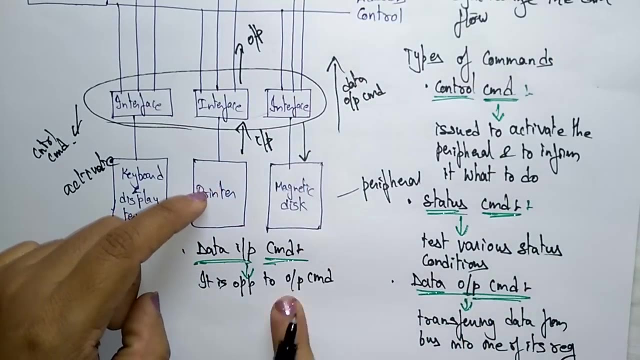 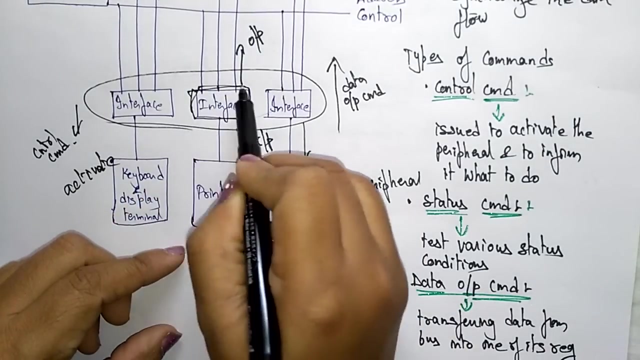 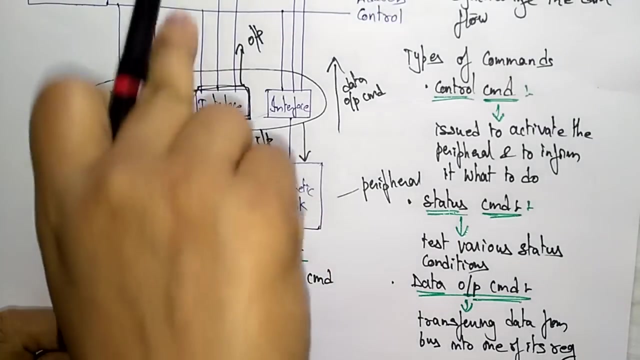 to the interface and here the output to the processor. okay, are you getting here? data output command is sending to the processor, whereas data input command is from peripherals to the interface. so the main focus here this is the interfacing circuit. so these interfacing circuit is having different types of commands will be issued to the processors as well as to the 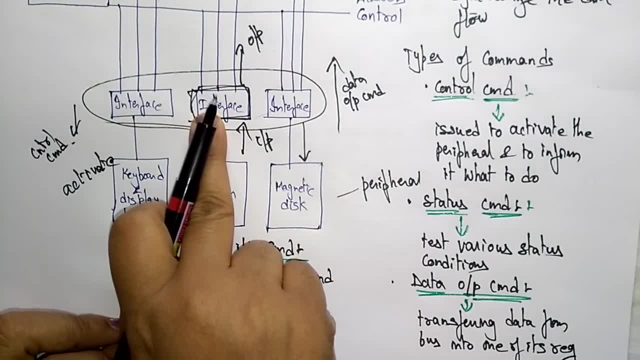 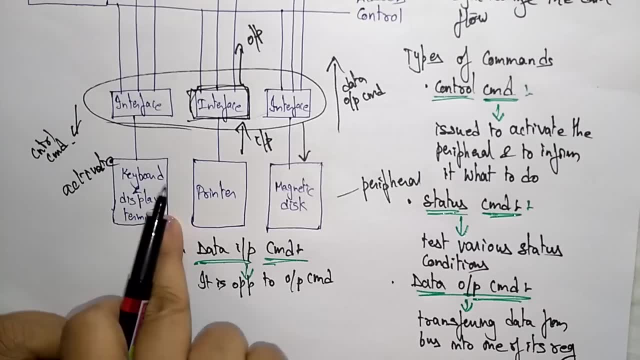 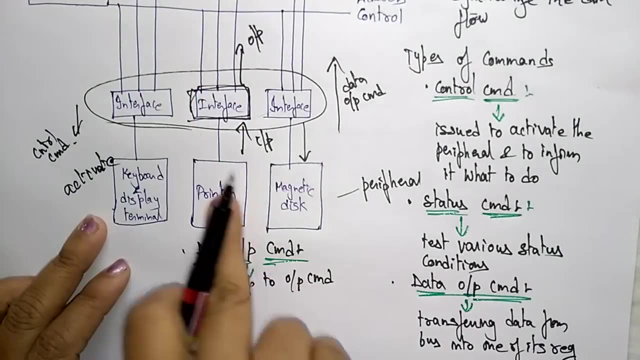 peripherals. okay, so control command. it sends a control to the peripherals: what, what, what, what it has to be done, what it has to be do. okay, so status command. so it's. it indicates the status of peripheral devices as well as the processor. okay, next is the data output command. so this is the data output command. it sends the 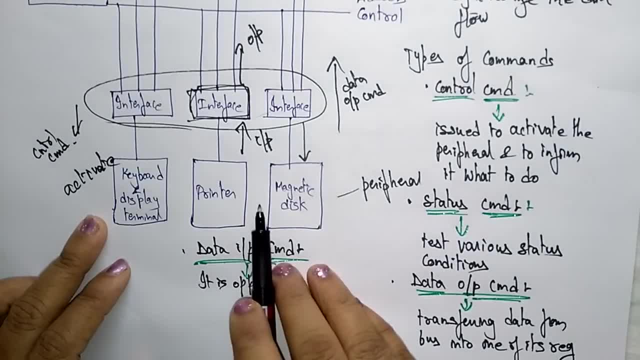 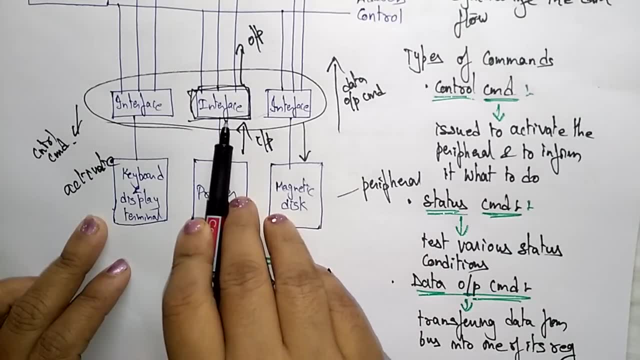 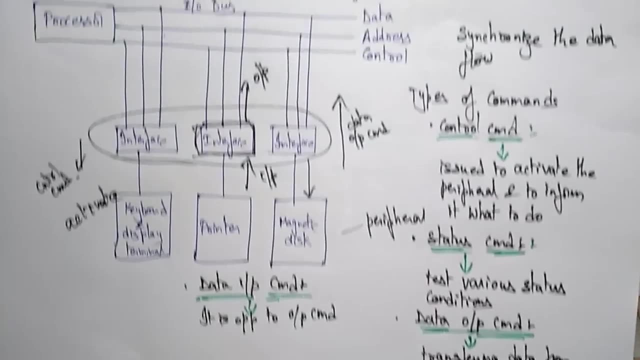 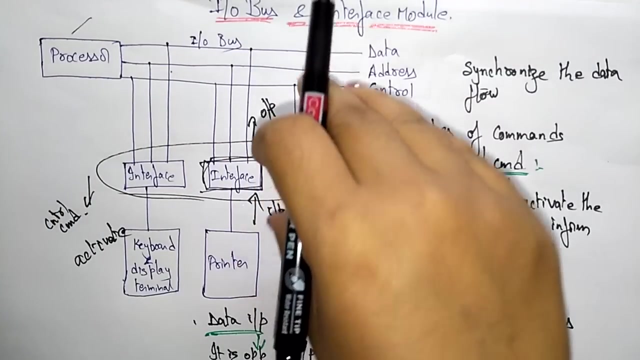 data to the processor and next data input command. so input from where this interface is getting, from peripherals. so from peripherals it is data input command will be sent to the interface interfacing circuit. okay, so this is the iobus in interface module. different peripherals and the processor will be communicated with the help of iobus and interface module. so let us see the. 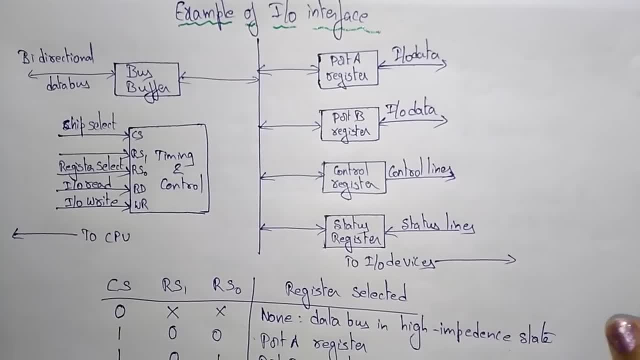 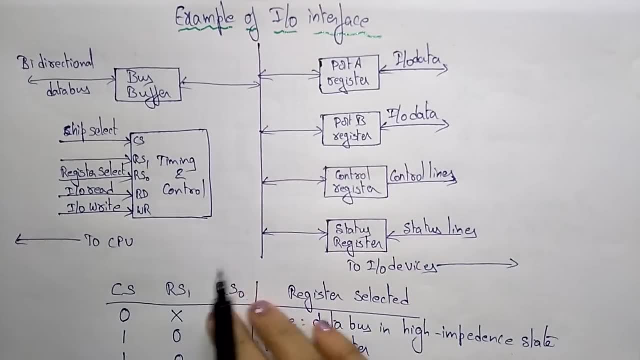 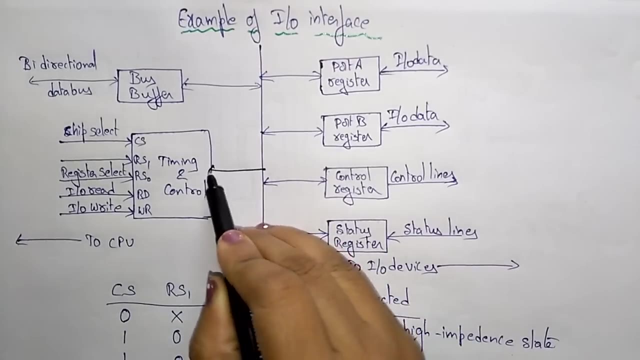 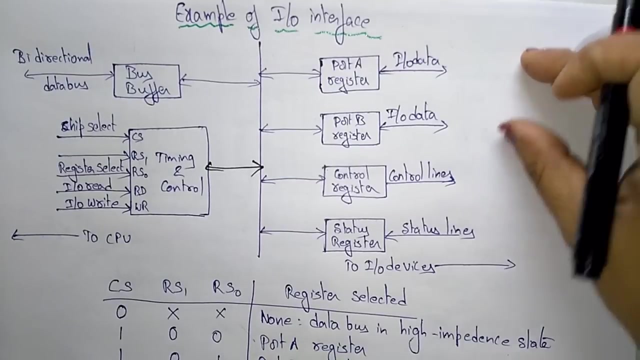 example of this ibo interface. so here you can see the example of ibo interface. so this ibo interface, this is a circuit and here this is the bus buffer will be there timing and control circuit and port a register, port b register. so these ports will be connected to the peripheral devices. okay, 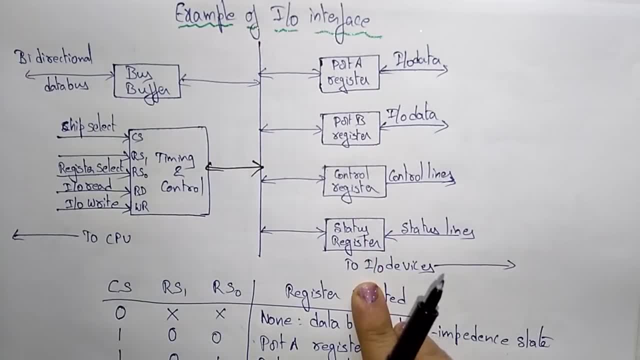 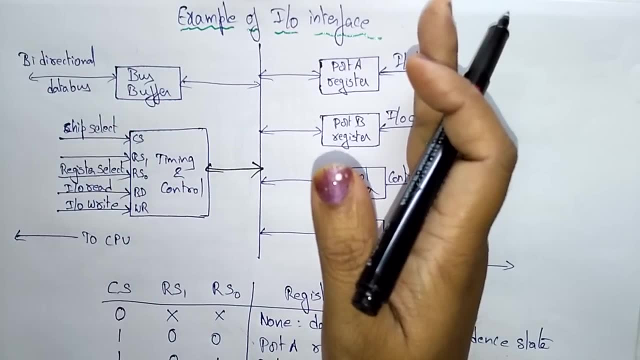 so, and this control register, status register. you have to be note that. so this is a interfacing circuit. this interfacing circuit, left hand side will be connected to the cpu, so all the pins here is connected to the cpu, and the right hand side will be connected to the cpu. so this is the 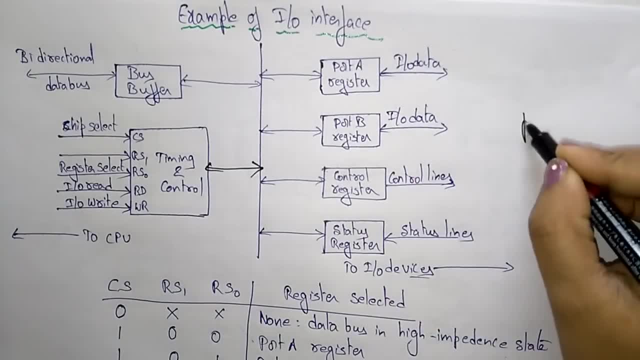 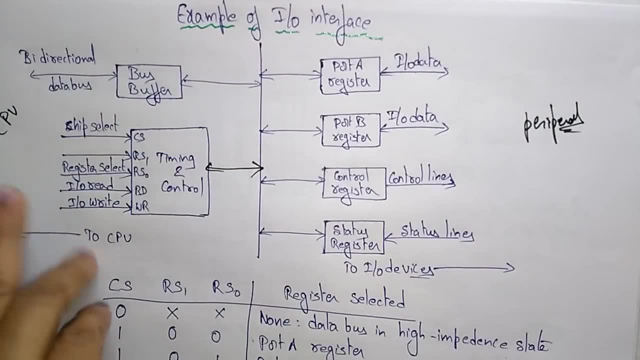 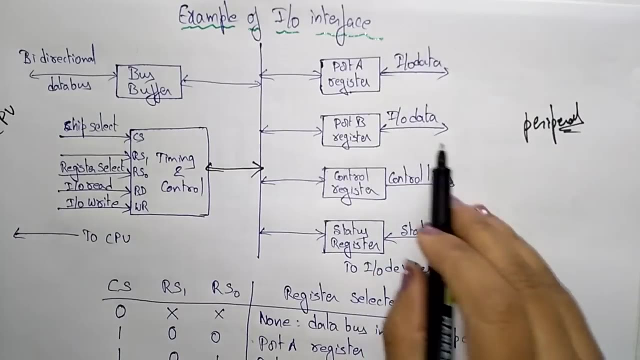 hand pins, all connected to the i o devices. so here the peripherals are there, here the cpu is there. okay, here the cpu and here the peripherals. so from peripherals you are getting the i o data and placed in the port- a register, and i o data input, output, data that 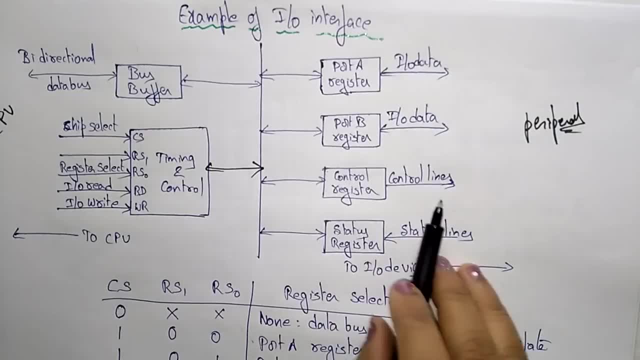 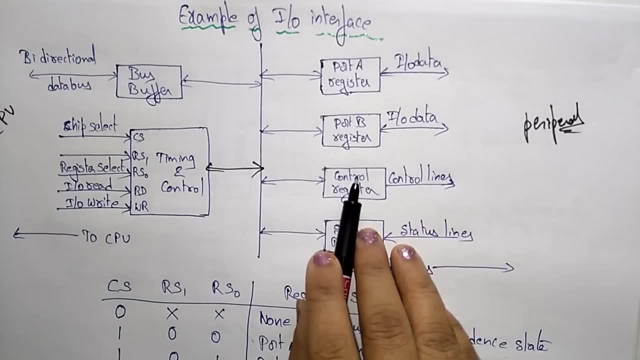 will be placed in the port b register. okay, so, and the control lines, so to where the data has to be transferred. every information regarding the control signals will be placed in the control register and the status of the each registers, or the status of the peripherals will be stored in. 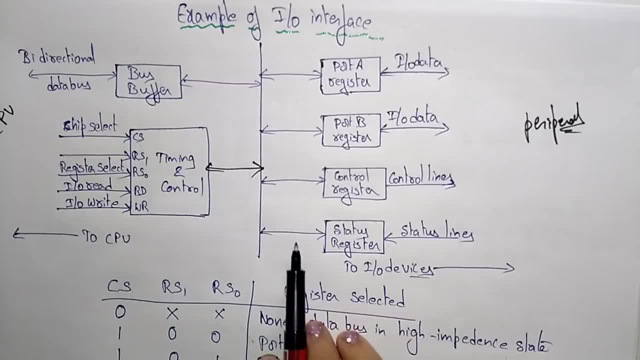 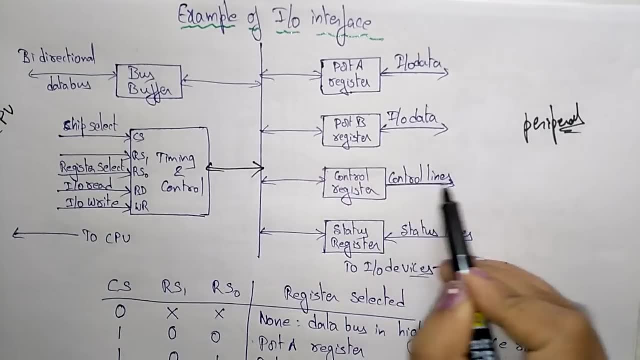 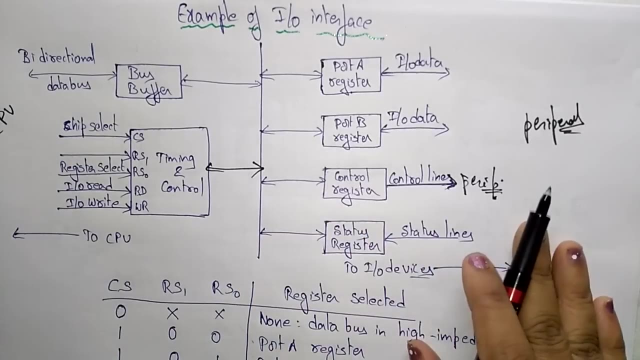 the status register. okay, so here, uh this: control lines are the unidirectional and the status lines are the? uh unidirectional, so control lines will be passed to the peripherals. why it is sending to the peripherals? because the cpu has to be uh send the signals to the